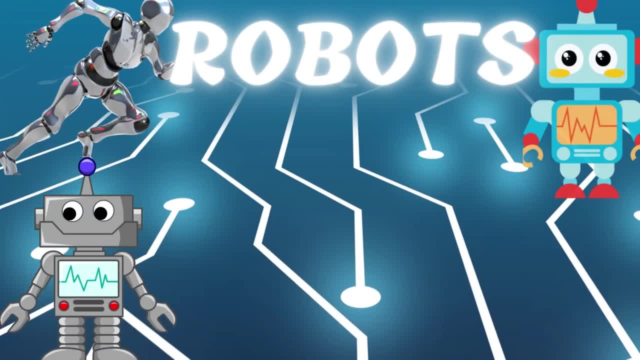 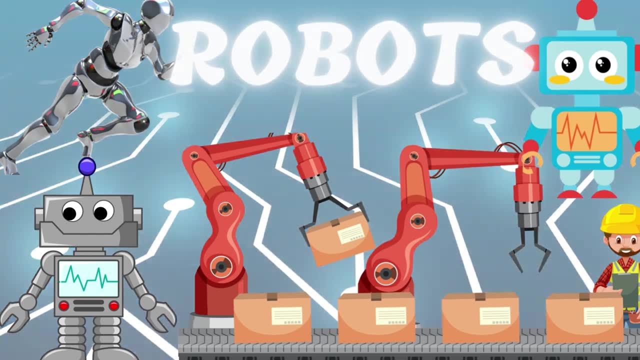 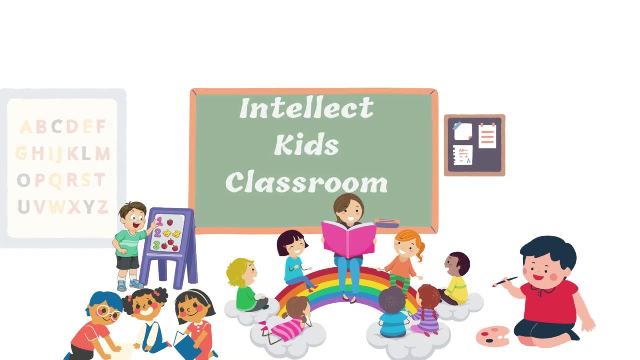 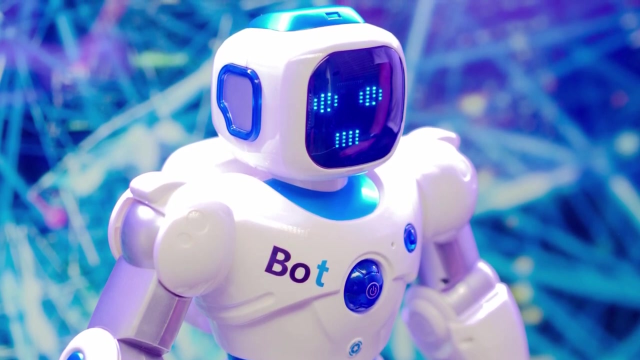 10, 9, 8, 7, 6, 5, 4, 3, 2, 1 0.. Hello kids, Welcome to Intellect Kids Classroom. Today we will learn about robots and the different types of robots. Robots are machines designed to perform repetitive tasks automatically and independently. 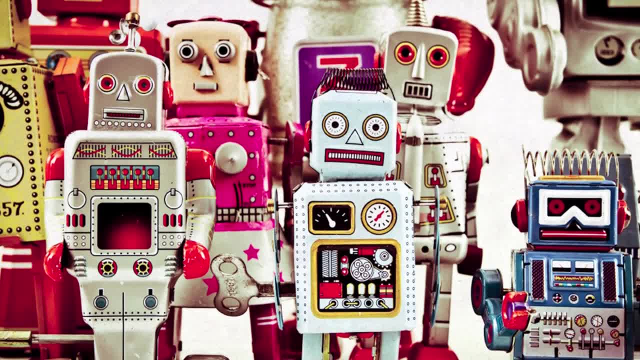 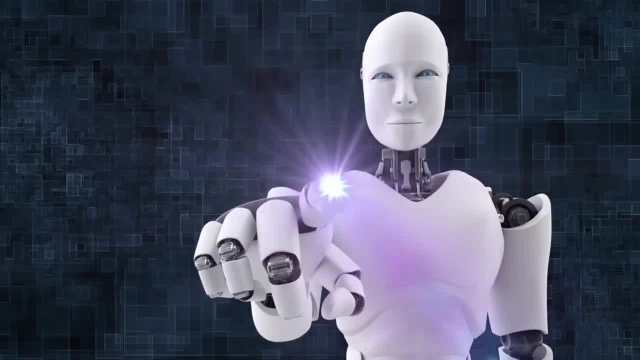 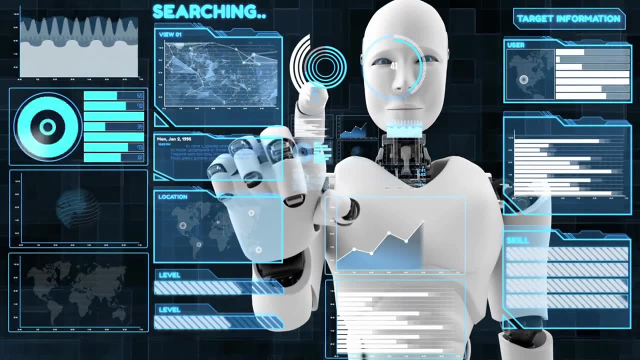 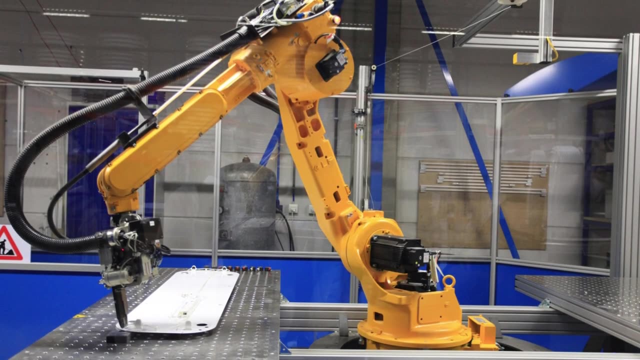 They come in various shapes and sizes, ranging from small toys to industrial machines. Most of us think that robots are used in the computer or IT industry, but they are also used in many other industries. Let us see some of them. Robots in the form of big industrial machines are used in the manufacturing industries. 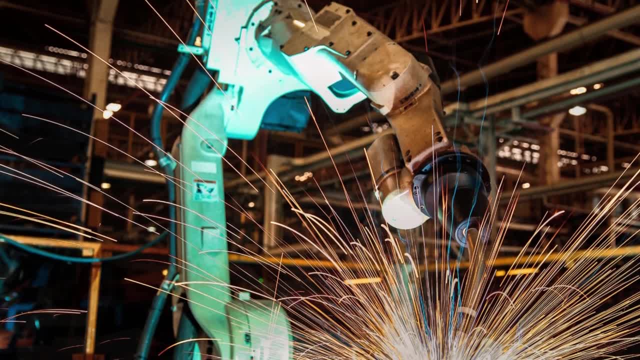 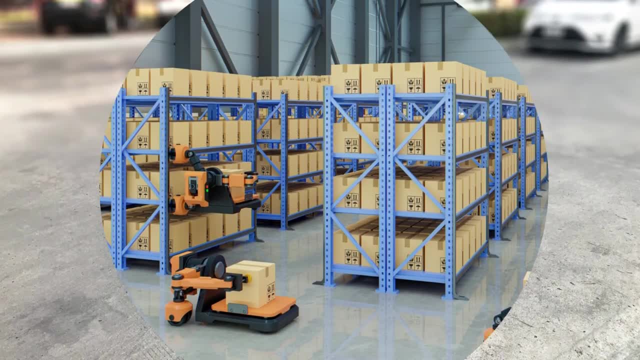 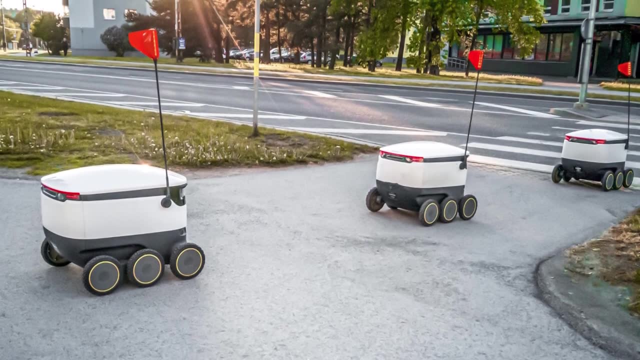 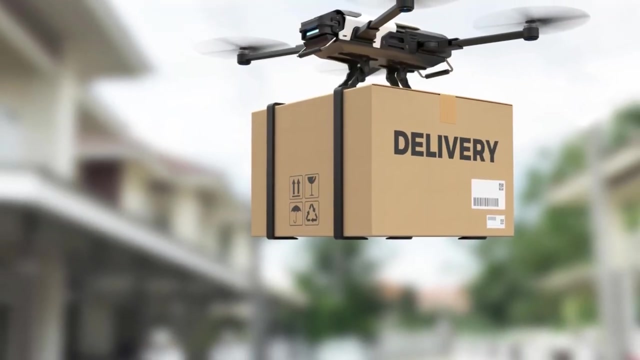 They can work in sensitive and hazardous environments. Autonomous robots are the robots which work independently in packing, shipping and delivery of products purchased online. In the near future, drones will be used to deliver packages. Some robots work in collaboration with huge companies. Some robots work in collaboration with huge companies. 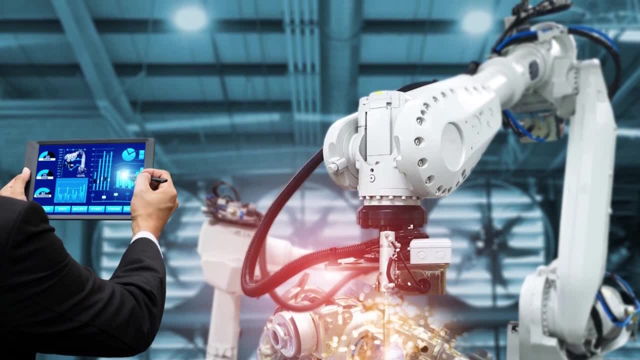 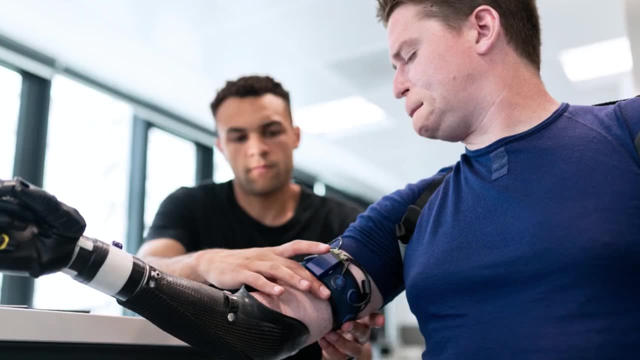 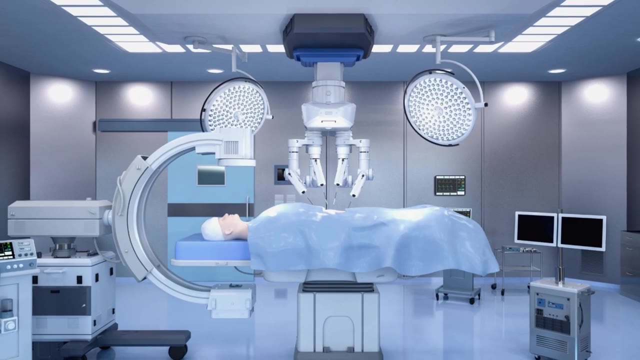 Some robots work in collaboration with huge companies. Some robots work in collaboration with humans to perform complex tasks. They are also known as cobots. With the developments in healthcare industry, robots are being used in surgeries and patient monitoring, etc. Robots are also designed to assist humans in tasks such as washing. 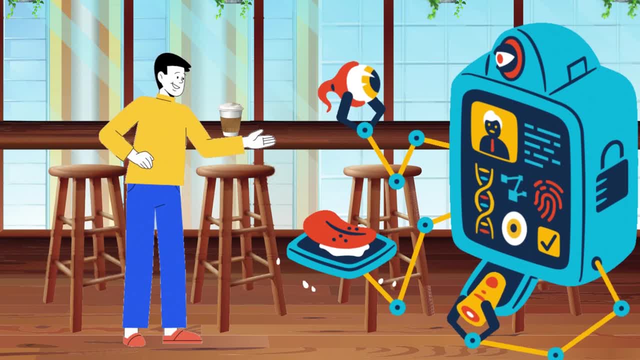 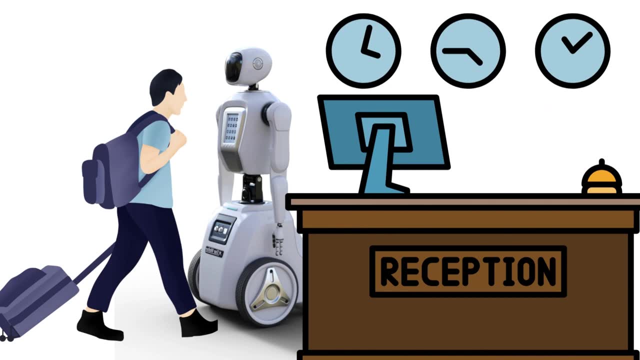 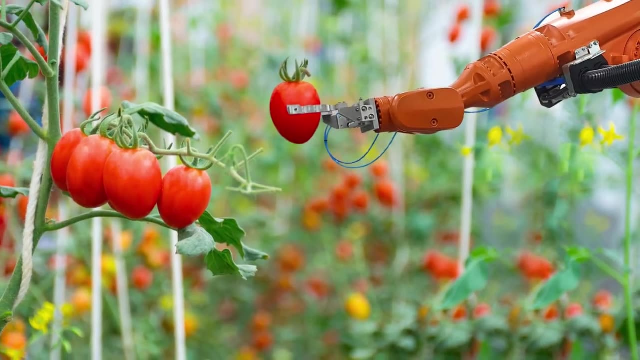 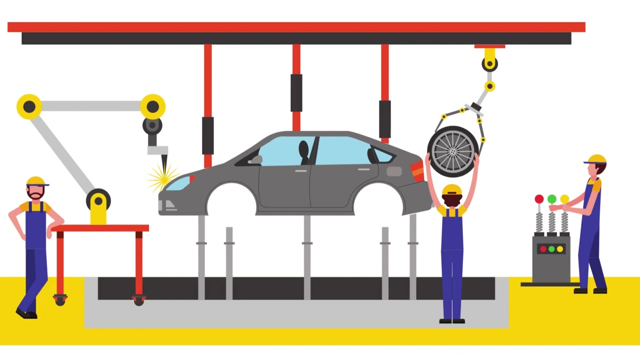 cleaning, cooking delicious food or providing customer service at hotel receptions. These are also known as servicebots. Agricultural robots are designed to use in agricultural tasks such as harvesting, planting and monitoring crops. Robots are widely used in car manufacturing industry in lifting, assembling, painting of cars.